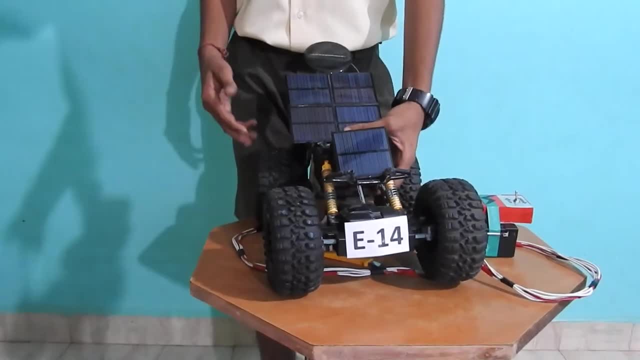 Topic of my exhibit is an eco-friendly vehicle. I have made a solar car by using these six solar panels, a 6 volt rechargeable battery, an on-off switch, forward-backward switch wires, motherboard and a battery. It can be used to run the motor.